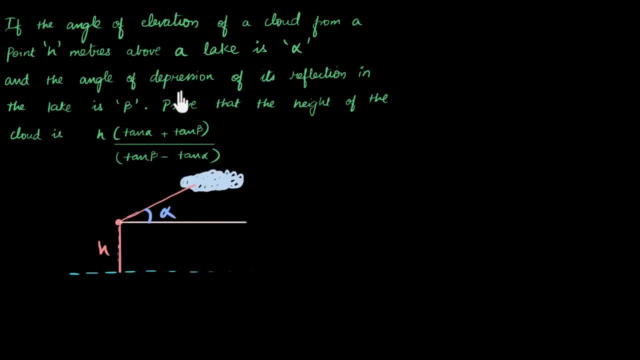 And my ability to draw diagrams. Quite a few things are coming together over here. So the angle of depression of its reflection in the lake is beta, Prove that the height of the cloud is something. Okay, I'm assuming the height of the cloud is the height from the lake, right? 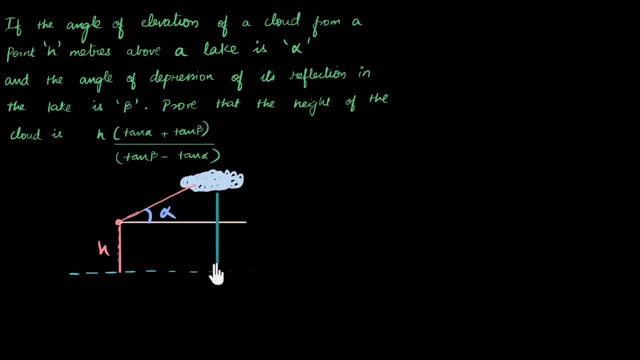 The overall height of it that it has from the lake. I'm going to mark that over here. That's what I need to prove- is equal to something, And I'm going to call that, I don't know, my x- This is what I want to find- Or my capital H, So that. 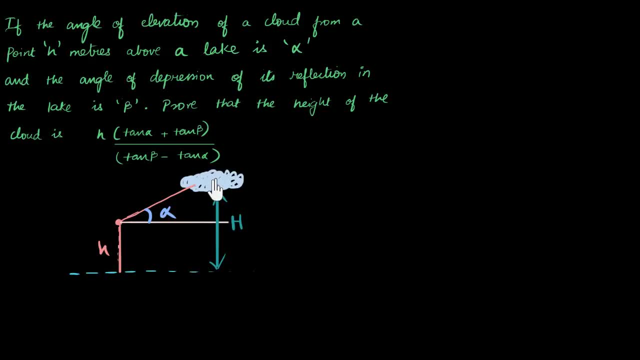 it still means height, right? So I don't forget that. Now, the thing about reflection: Now I feel I'm using some physics knowledge here, So I'm wondering if I'm interpreting the question correctly. The thing about the reflection is that that will be formed exactly at the same distance. 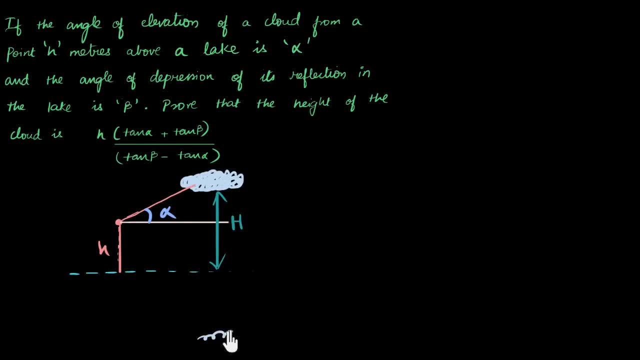 on the other side, assuming the lake is like a plane surface, which is, which is, a fair assumption. So I have my reflection somewhere over here And the only thing I know about this reflection is that the distance from the lake to the reflection will also be h. 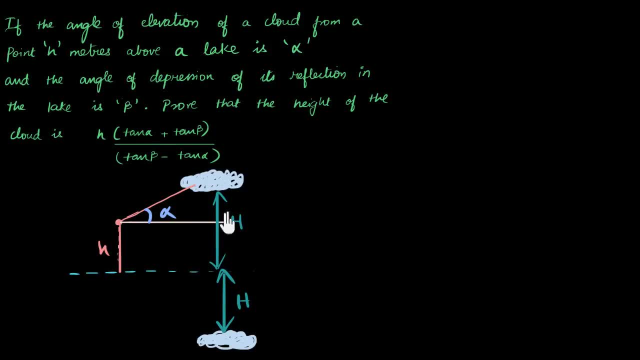 Okay, This is actually a pretty interesting question. Okay, So these two are h. They may not look exactly the same in the way I've drawn it. I'm trying to stay within the frame And what's told to me is that the angle of depression of its reflection in the lake is beta from, I'm assuming 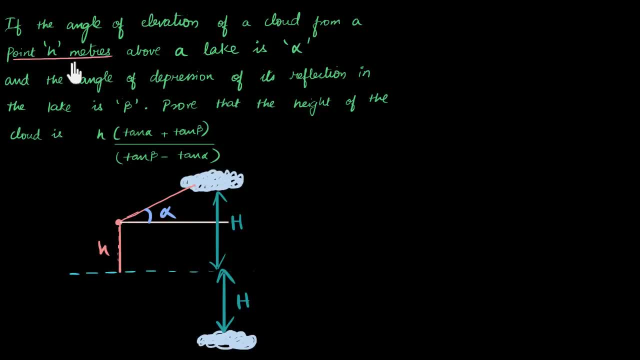 it's from the same point. That's h meters above. It's from this same point, So let me draw that the line over here. Okay, So arriving at the diagram is usually the part that needs a lot of work. So I think we are almost there right now. I think this angle let's use a different. 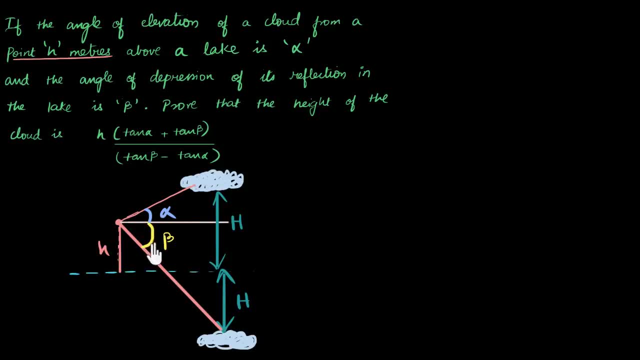 let's make it yellow And this is beta. So we have the diagram And I think that's all the information that we have. We've used everything. Alpha has been used, Beta has been used. Point h- meters above has been used. We have to find the overall height. We're calling that h. Now we have 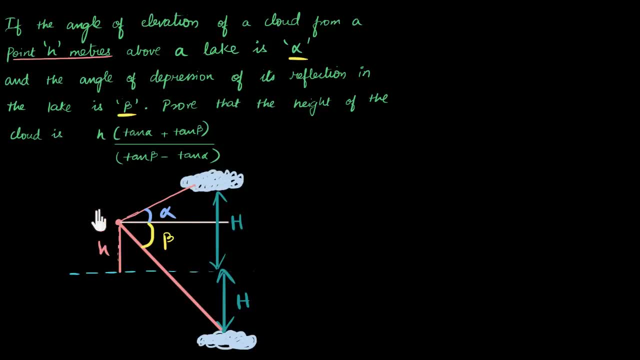 to show that this capital, H, equals this thing that contains h, alpha and beta. Okay, I think I'm ready to go. You can like, if you, if you want to, you can try this on your own and see how the graph looks over here, to try and write some equations that connect these. What do I see? I see. 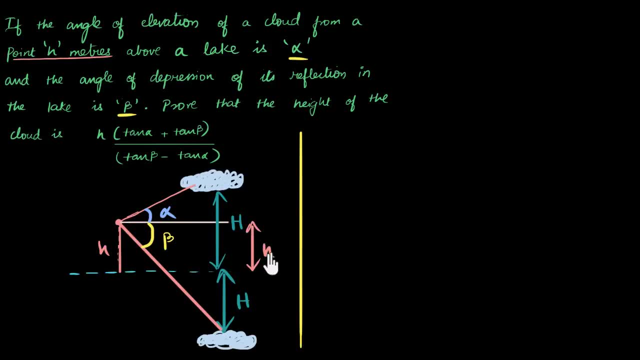 that this also has to be h. This length has to be h, So this gap over here is capital H minus small h. The reason I'm trying to find this gap is that I'm I'm seeing all tan alphas over here, but for 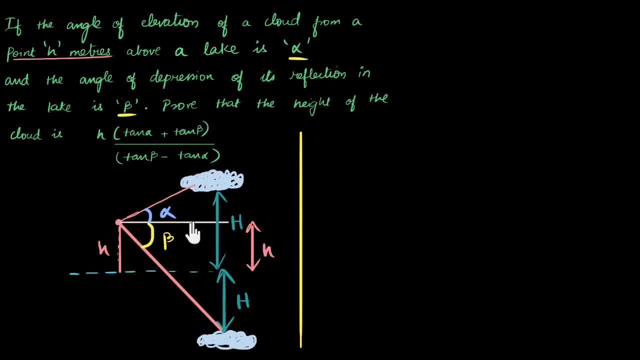 tan. I need this side, right, Opposite by adjacent, opposite by adjacent. So I'm thinking: how do I, how do I bring these into my expression somehow? I have to try and work my way to this. I have no idea how. I'm just going to try, Um, and hopefully it won't be, I won't make. 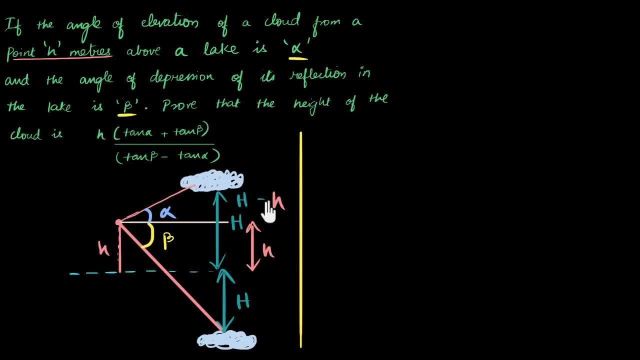 too many mistakes and I'll. I'll somehow get to the answer in in the in a, in a short enough path. Let's hope So. capital H minus small h is this length. I'm going to take this length as something It's not given to me, So maybe I'll just take it as some d? Uh, I'm going to write. 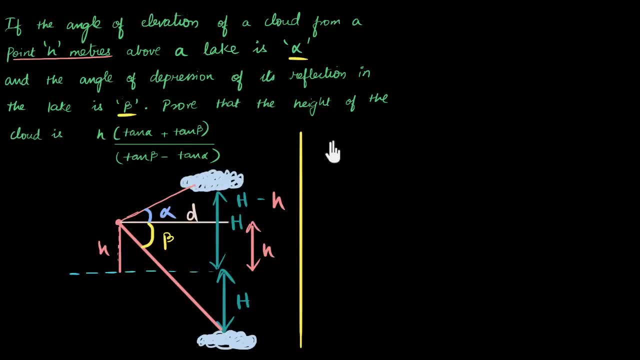 my equations and see what happens. right, Because I want tan alpha, I'm going to write: say, tan of alpha now equals h minus small h by d. Would you agree with that? Just look at the diagram And opposite by adjacent. So you will agree with that by d. Now what is tan, beta, Tan? 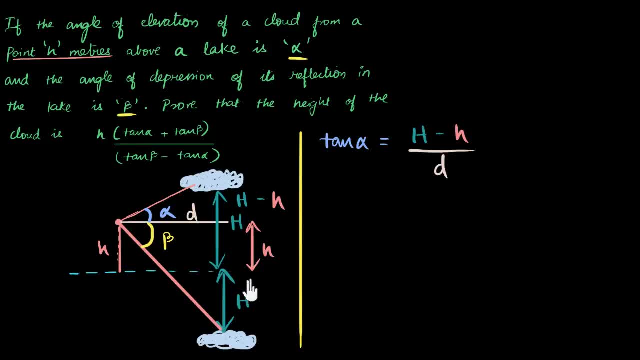 beta is uh, uh, small h plus h, because this gap over here is this bit over here is capital, H minus small. sorry, it's just small h, It's the same as this length Plus I have another distance, a depth into the uh, into the lake, where the reflection forms And the key idea. 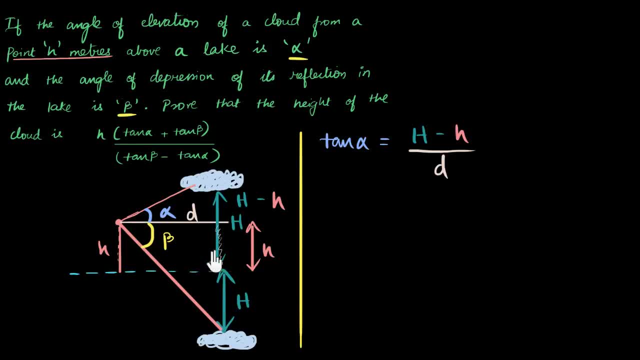 that we had from physics was that this height h and this height h will have to be equal to the same. That's what we mean by reflection. So it's also a mini physics question. So then we have tan beta. Tan of beta equals h plus h. That is small h plus big H by d, Let's. 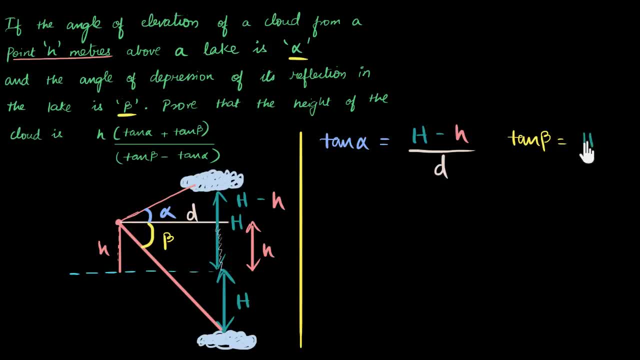 write that Um h plus. I'm beginning to feel a little bit optimistic, actually, because I see some patterns emerging over here by d. Now I know what I don't need. I don't need d, Nobody cares about it. So I can try and eliminate d. I have two equations. Uh, how many variables. 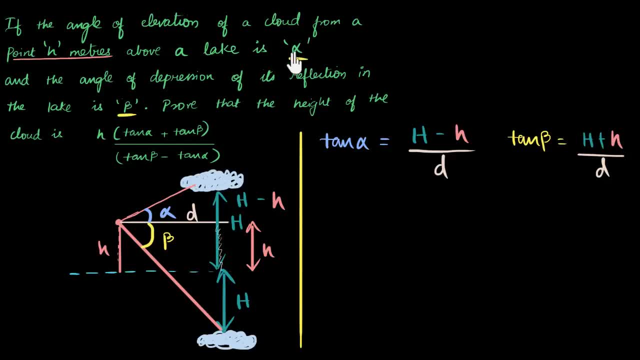 do I have? I have two variables, because alpha is not a variable that's given to me, Beta is not a variable that's also given to me. Um h is also given to me, small h. I should have named it x or something. I'm just like. that would have made it much easier for me. 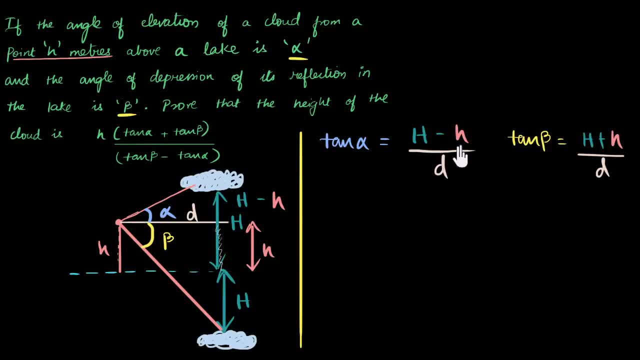 to refer to h and x and all that. It's fine, Bear with me. And d is not given, So I'm using the word variable a little loosely here. What I mean is that there are only two things here given in the question that I assumed, that's capital: H and d. The others, all of the others. 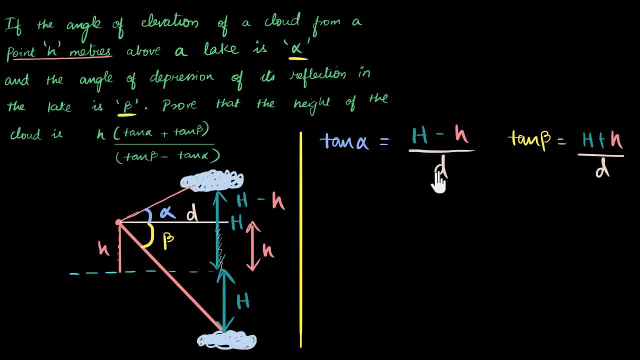 were given as part of the question. So there are two variables here. capital H and D are the variables, Rest all are given. So two variables, two equations. I know I can solve it. Whether I can reach this form, Let's see. that might require some, some skills that. 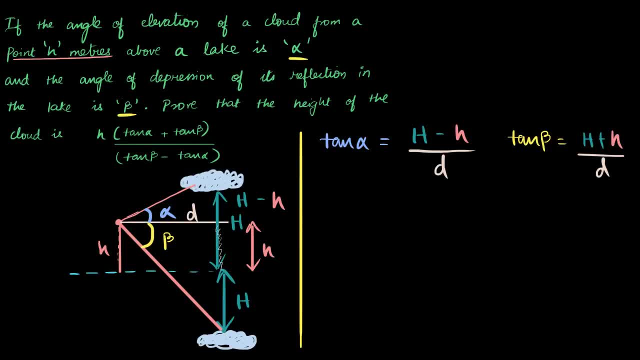 I may or may not have. Let's see where. eliminate d So um. let me do that. So from this equation I can write d as h minus h by tan alpha. So d equals min d. Now when I do this, what's? 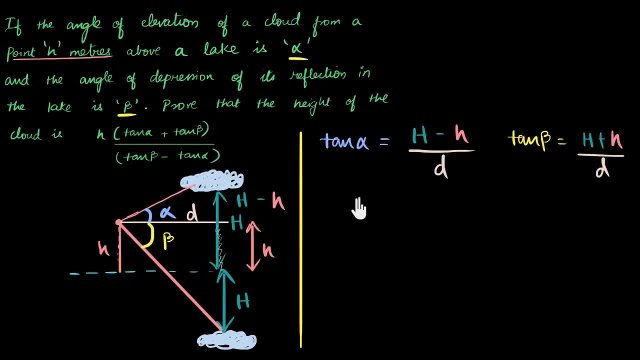 it gonna do. It's gonna go this way. Let me go back to the first step, which is always part of the equation: Um. so let me uh deselect d, Uh, and then from this equation I can write tan alpha. so d equals H minus h by tan alpha and that will be equal from this one here. 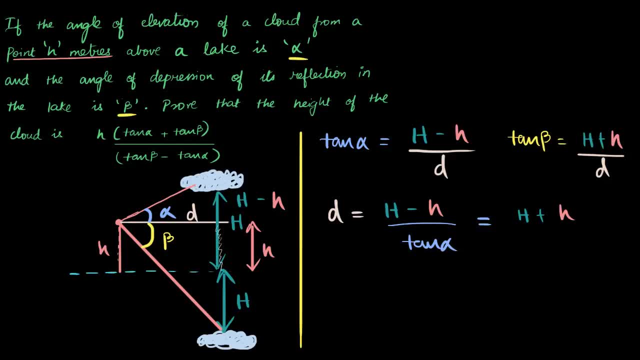 capital H plus small h by tan beta, by tan beta. Now I have one equation which contains all the variables I need, and my hope now is that I can rearrange them and get it in the form that I want. I have to take my h out separately. 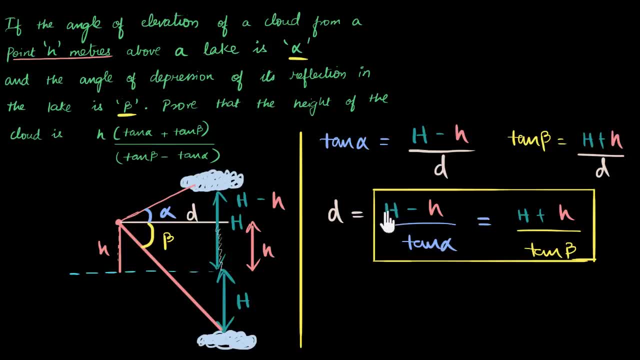 So I'm going to cross multiply first. So that will be capital H tan beta minus small h tan beta. on this side I'm going to write that So capital H tan beta minus small h tan beta, tan beta or beta- how is that pronounced? 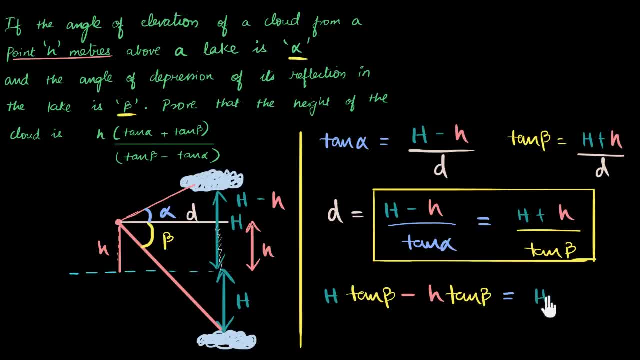 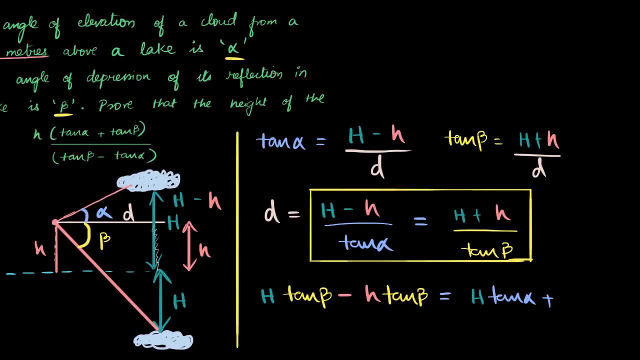 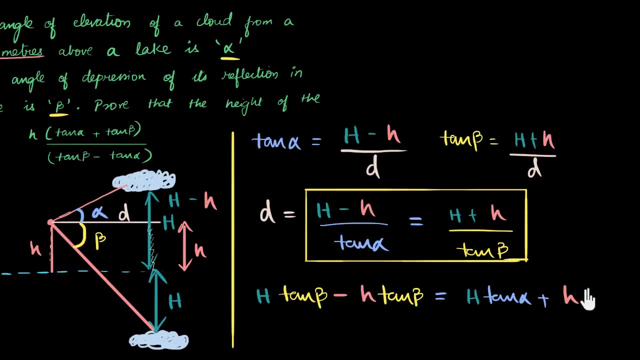 And capital H tan alpha, Capital H tan alpha plus, and I'm going to make some space plus small h tan alpha, Small h. I actually feel that we're going to reach the answer very soon, because after this it just seems like I can take this to the other side, take that to the other side, divide. 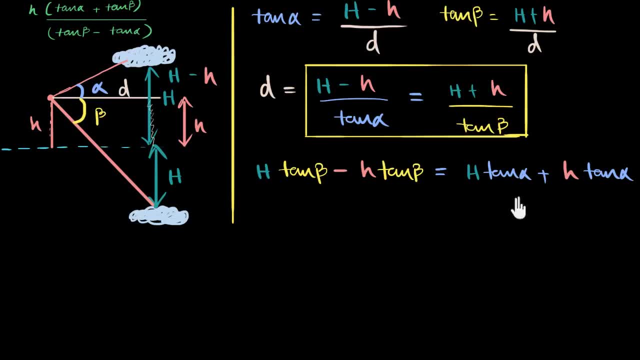 and I'll have my answer. You can almost see it right. It's tempting. So I'm going to subtract both sides with capital: H tan alpha. So I'm going to subtract both sides with capital H tan alpha. So if I do that, what I'll get is H times tan beta minus tan alpha, tan beta minus tan. 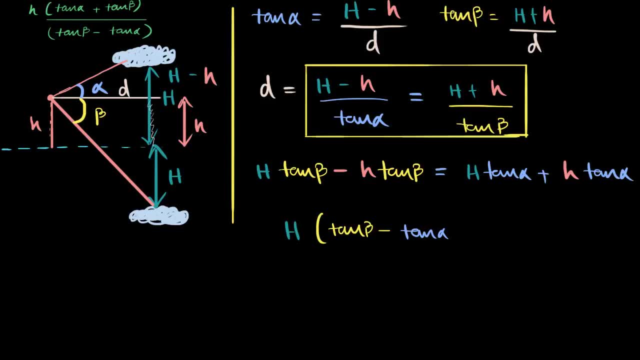 alpha, tan alpha, And that'll be equal to. I'll add h tan beta, small h tan beta to both sides. Then I'll have the. it'll go away over here, And over here I'll have small h times tan alpha plus tan beta. 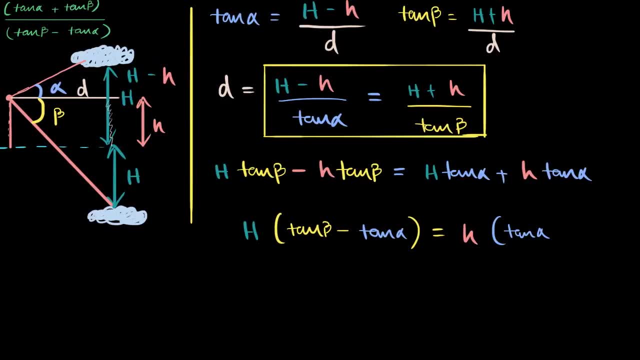 So tan alpha plus tan beta- Okay, Plus tan beta, And that is it. Now I have to just divide both sides by tan beta minus tan alpha and I have what I want. So let me write it over here: H equals- yeah, I'm excited. 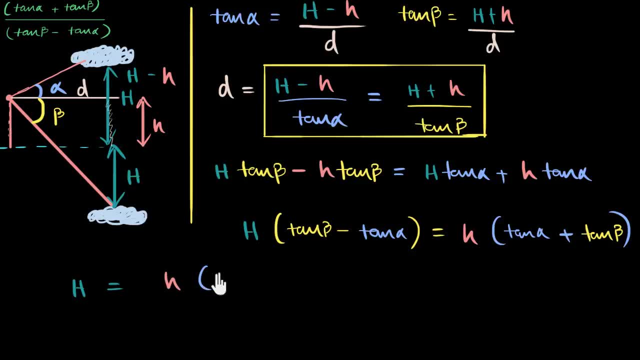 This is. this is nice, This is. this happens sooner. I got the answer sooner than I thought I would. Tan alpha minus- sorry, plus tan beta by tan beta minus tan alpha. Tan beta Minus Tan alpha. And there it is. 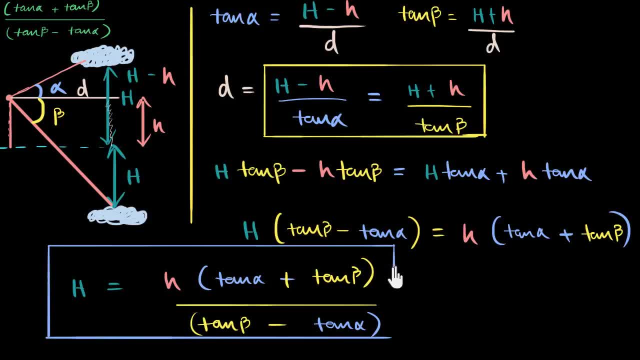 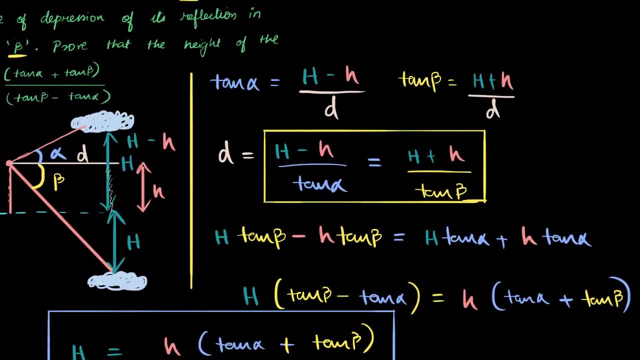 Whenever I get a nice result like this, I like to put a box around it And let me check if this is what was in the question. by the way, tan alpha plus tan beta by tan beta minus tan alpha- Awesome, So it is what I wanted. 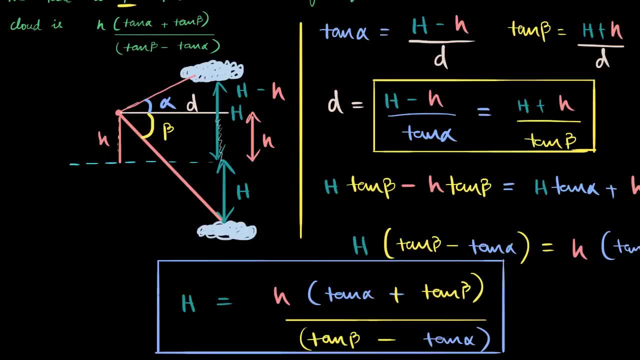 So let's bring it all back down over here And there we have it Now. because it's a proof question, I may not want to like maybe dig too deeply. I'm pretty sure I've got the right answer, But if it wasn't a proof, if I had got this, I'll try and look at a few things. 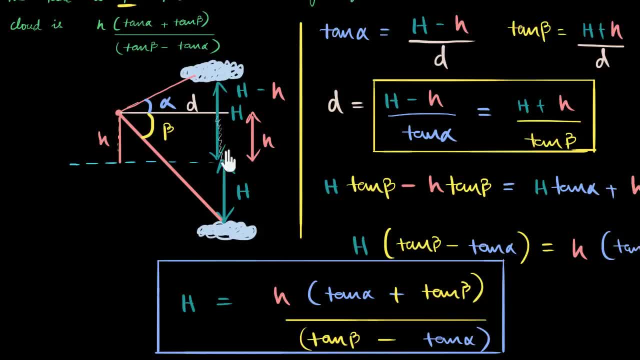 I'll look. maybe hey, can this denominator be zero. In other words, can beta ever be equal to alpha, And that's. you'll notice that that's possible when H equals zero, When H becomes zero, only then that'll happen. so that's like an edge case over here. 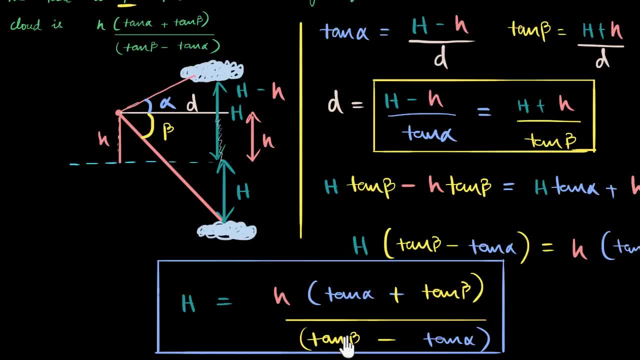 I'll try and understand. okay, for every other case, where H is a positive number, beta will be larger than alpha. So tan beta will also be larger than tan alpha. So I'm checking basically if this height will be a positive number. right, because the way 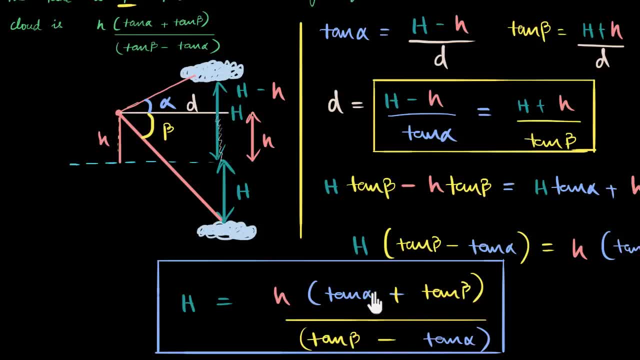 I've defined it, This height should be some positive number. I'm checking if this is obviously positive because both these angles are acute, So this will be positive. This also will be positive as long as the height H is positive. Now I'm curious if I make my H negative, if there's some fish watching this, what would 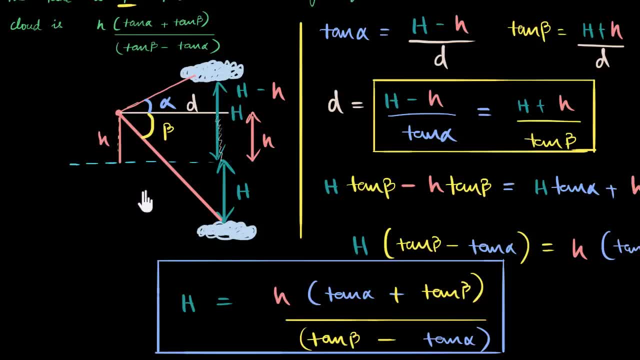 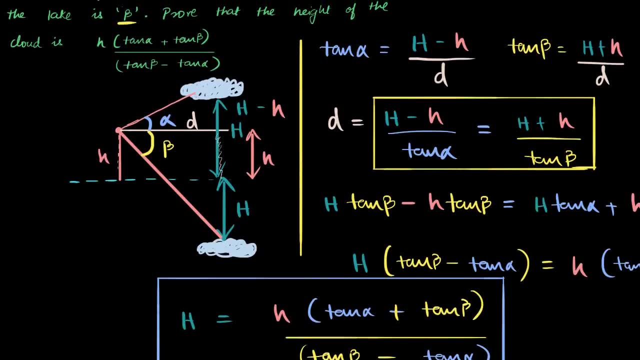 happen to my scenario. That's a good excursion that you can think about, But if you notice, all the questions that you've done till now basically boil down to taking the story that was given to us. this was a story- And drawing a diagram. 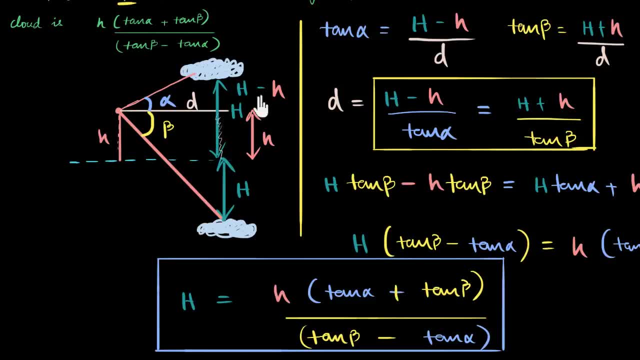 Like we did over here, And noticing the right angle triangles, asking where are the right angle triangles? And noticing that there's one here. maybe I should complete it over here- Yeah, that right angle triangle and this one over here, And then writing equations that connect the quantities that are given to you to the quantities.